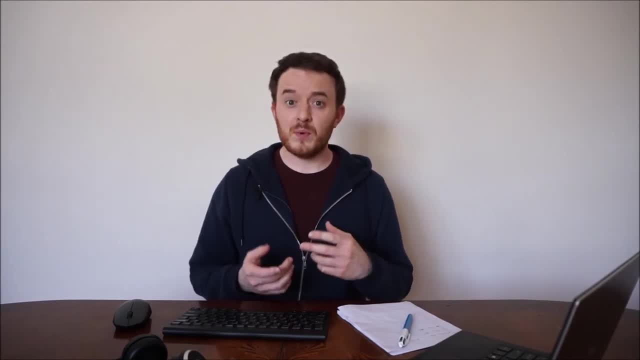 textbooks should be a great combination. So here on YouTube, we're making videos that are going to help you guys in terms of the content. If you want help with exam paper questions, mastering all the different techniques, then go over to our website, thegeographyacademycom, or to our Instagram account. 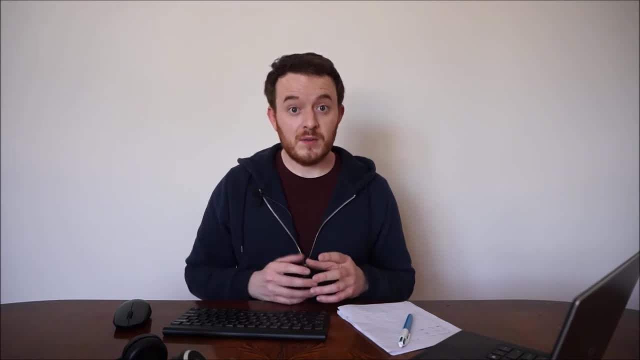 and have a look through what we have on offer there. So let's start off. We're going to start off by looking at farming systems in the different types of farming, and hopefully by the end you'll have a clear understanding of what differentiates each definition. Arable farming is the production. 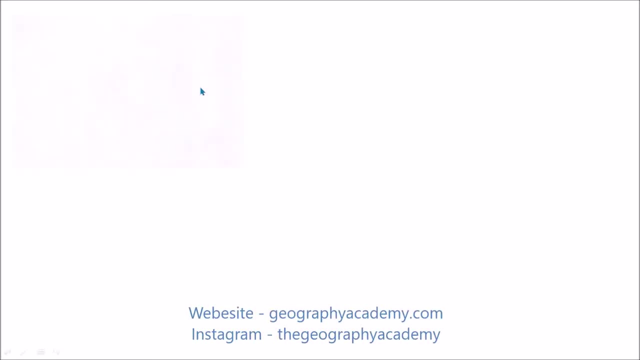 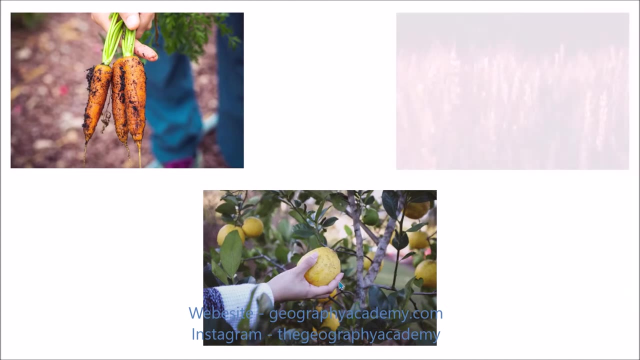 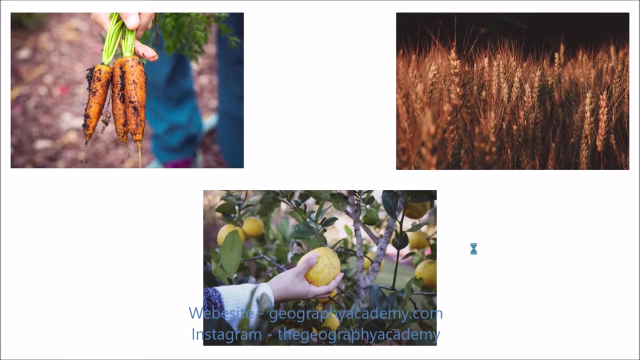 of crops. This might include vegetables such as carrots and our root vegetables, and we could get our fruits, and this includes our grains as well. So those are three types of food, and within those then are loads of variations of those foods: Arable farming, then, looking at any farming, it's all in a system. So we've got 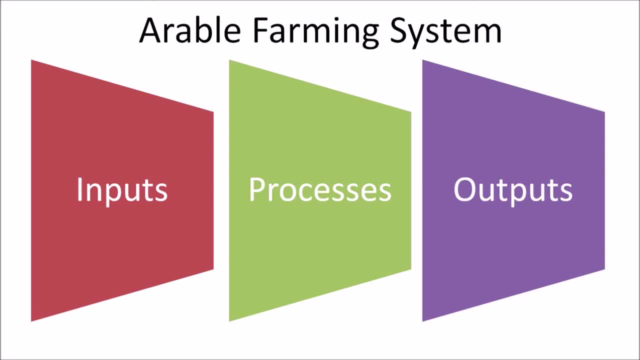 everything in a system: inputs, processes and outputs. Our inputs are what we need in order to begin. Our processes are the jobs that we have to do to help us produce the goods, like the vegetables in this case, and then our outputs, then, are going to be what we sell from the farm. 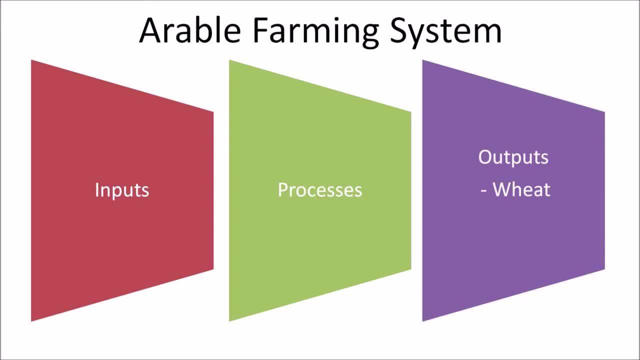 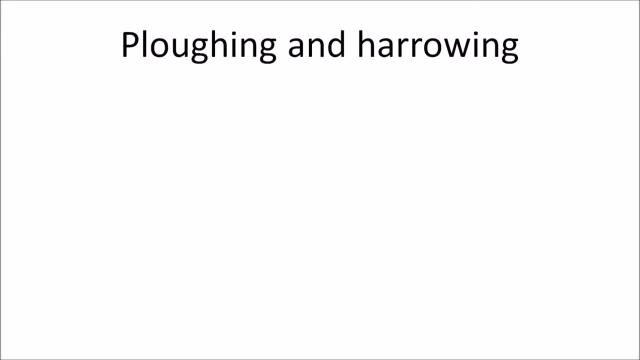 Arable farming system, we start with one output anyways. We can look at wheat as an example. Wheat has many processes and many inputs to it. So plowing and harrowing- Plowing- we need to turn over the soil. So the soil might look like this at the end of the growing season, after the crops. 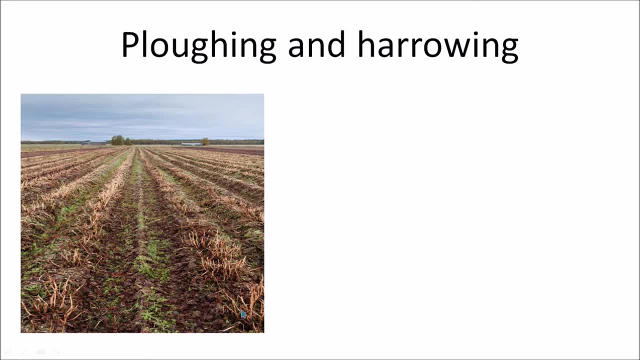 have been taken in and what we have are the roots from the previous crops, and we've also got our weeds that are growing up through the soil. So the idea of plowing is that we will turn over this soil and we'll send all the vegetables to the soil and we'll send all the vegetables to the soil. So 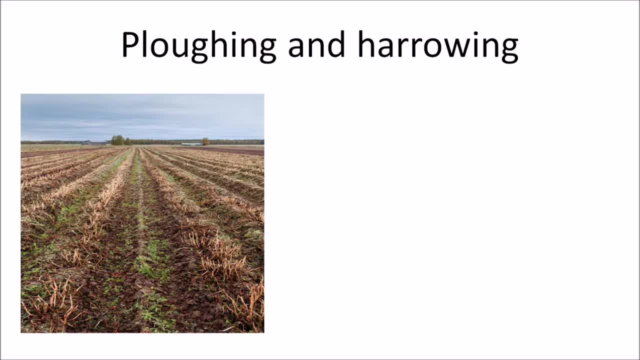 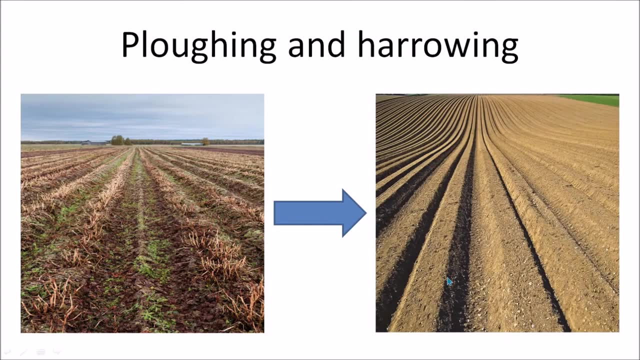 we'll send the vegetation down into the ground and this will add to the soil's fertility, and we'll also then straighten that out and make it nice and neat by harrowing, which is to make it into that very smooth texture, which means this soil is ready to be used then to grow crops. So those are. 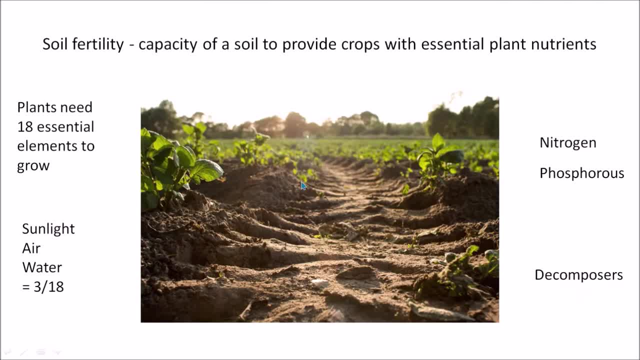 two processes there in order to get the field ready. Now, we might as well take this time to explain something, because it will be mentioned again and again throughout geography in different areas. So you will hear about soil fertility and that's the capacity of the soil to provide crops with 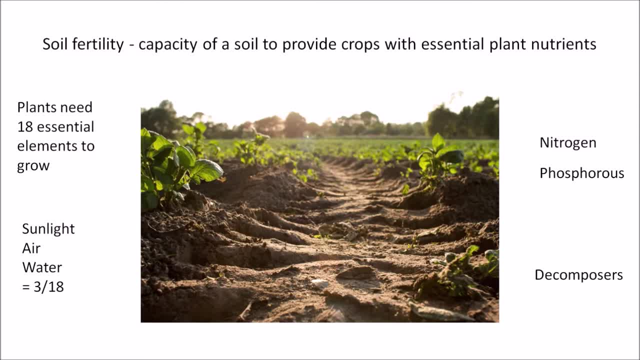 essential plant nutrients. So what do we mean by nutrients? Well, they're just different elements that the plant needs in order to grow: Now, from sunlight- and you know our photosynthesis- and the air and the water that the plant receives. that's about three out of 18 essential elements. 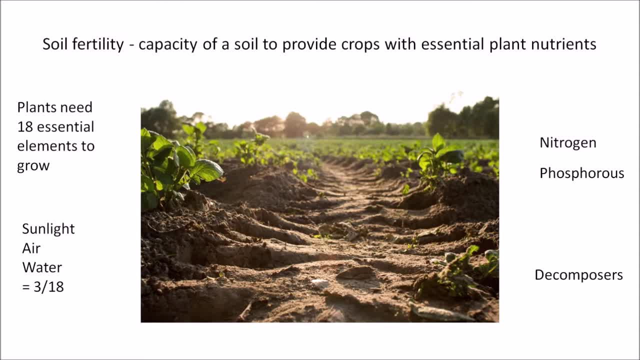 that a plant needs to grow. Some plants only need about 15.. So something that's quite commonly found to make up for the rest of those- let's say there's 15 left in this case. So we need things like nitrogen and phosphorus, and they're found in the soil because of things like broken organic matter. 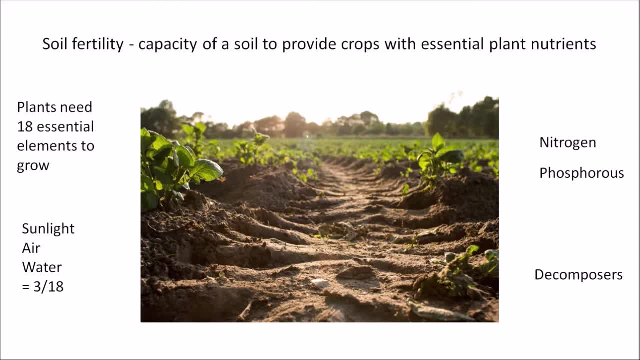 like those plants that we talked about being in the soil. when they're turned over, that organic matter will die and then the nutrients will attach itself to the soil and then the plant can use this later, Decomposes then within the ground like things like our worms or moles and things that can either eat. 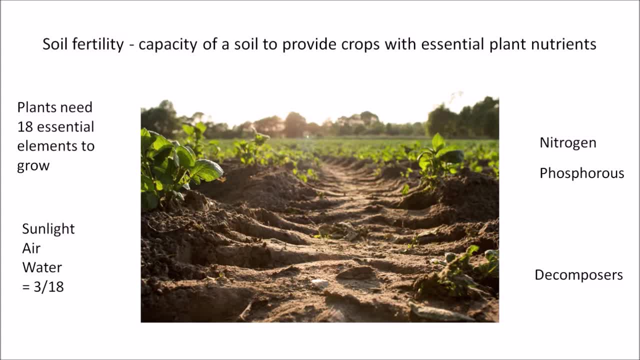 organic matter, or they die themselves, or they just mix it around and help to break it down. So this is. these are all components of a kind of healthy, fertile soil. In doing so, then, we've got enough of these elements that can provide the food with all its nutrients in order to grow. Weeding. 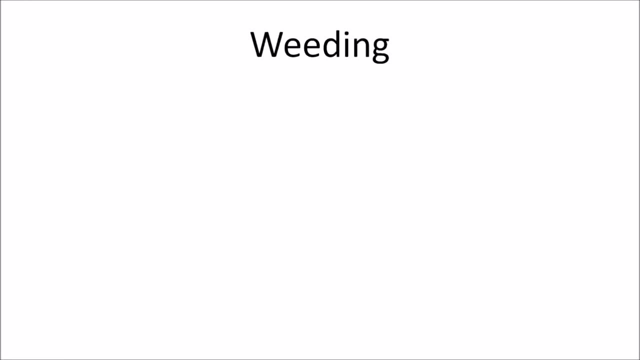 then we've got to look after the soil. So before and during the growing process of the wheat, it might- you might see a lot of weeds starting to grow up Now. these are not good in arable farms- in most farms- not well. they could add things like your nitrogen and phosphorus to the soil. Yeah, 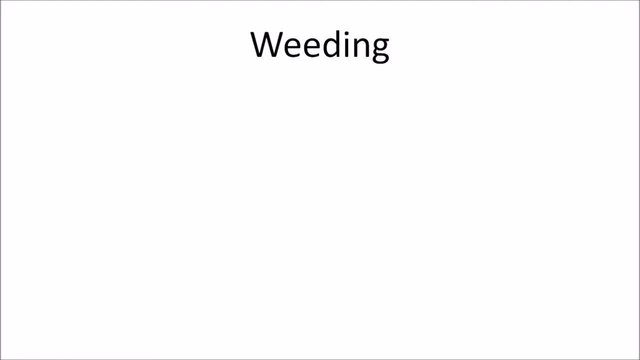 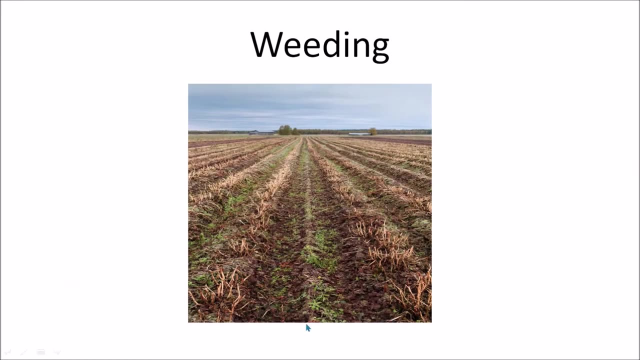 sure, But they can also outcompete the crops, such as the wheat for all its essential nutrients. So for weeding, we really want to get rid of all this sort of stuff in the middle here and make sure that our soil is nice, plain and that there'll only be one primary plant growing in that area. 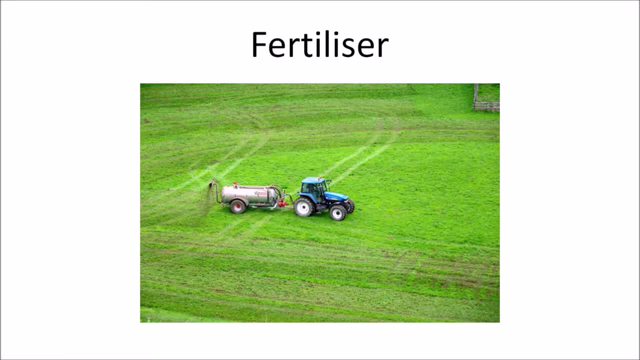 Fertilizer, then, is an area that we can do this organically, which means that we might use natural fertilizer, like this gentleman here is spraying some manure onto the fields And this is instantly fertilizing it by giving it all those essential elements like the nitrogen and phosphorus, into the field. So this can be. 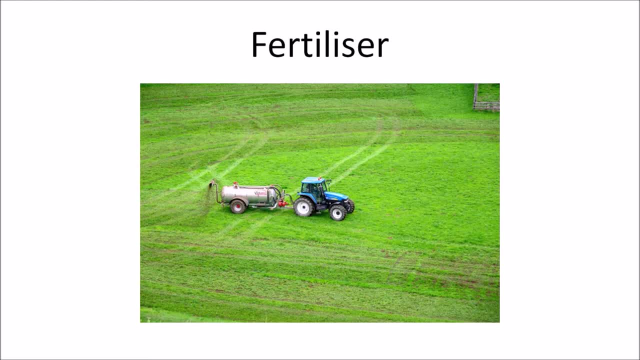 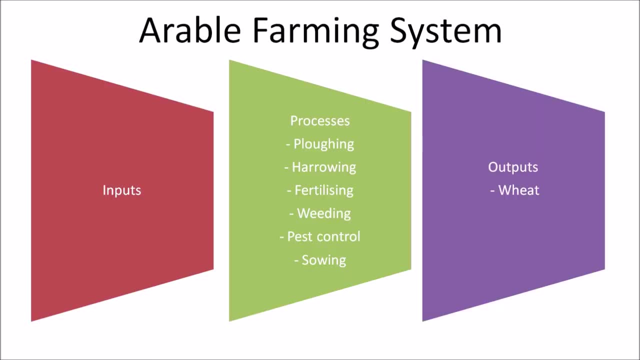 done organically, like this, or inorganically, where we can get a chemically produced fertilizer that might add a specific amount, of say, nitrogen or phosphorus. So, yeah, that would be our process, And that's it for this video. Thanks for watching And I'll see you in the next one. 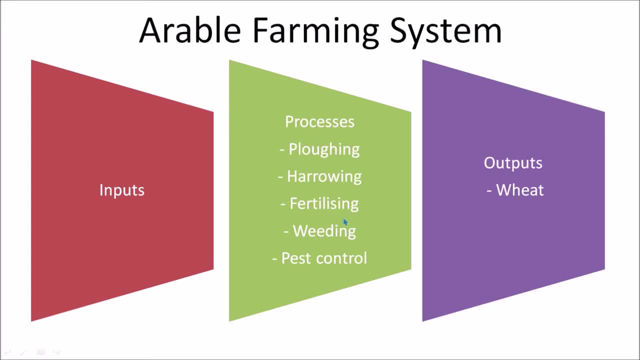 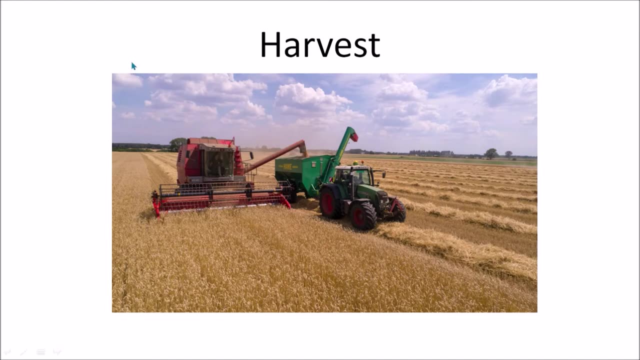 Bye machine, And this is actually quite a useful one, the combine harvester- because it's got to go through the processes of reaping, threshing and winnowing. So essentially it's dividing up the pieces of the crop and then it's putting them in and organizing them up. So this would be an 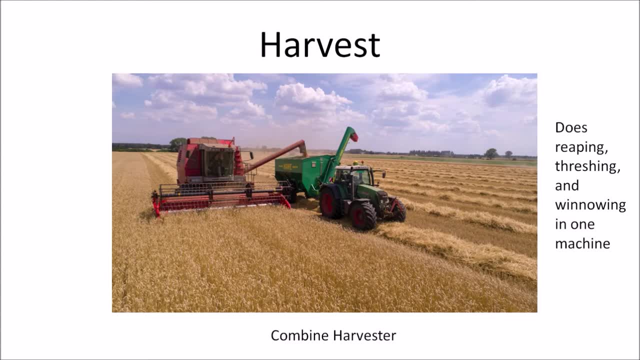 example of machinery making things very time efficient And also like saving like three jobs into one. And if you had something on this scale, you couldn't do it with just two people driving a machine, But you would need a huge quantity of people working in that field around harvest time. 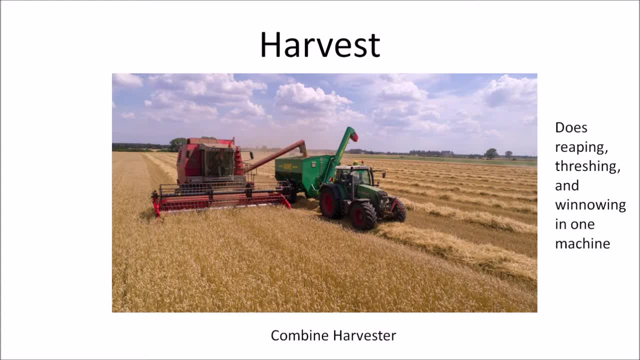 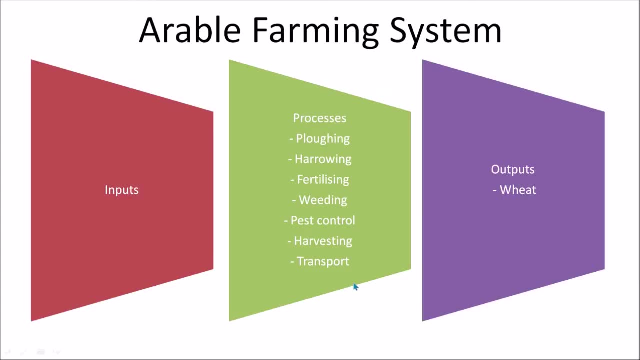 which traditionally happened and still does happen around the world. But if you've got machinery, in this case for, say, harvesting grains, it's very, very efficient, All right after harvesting- then you've got to include our transport too, So that could be. 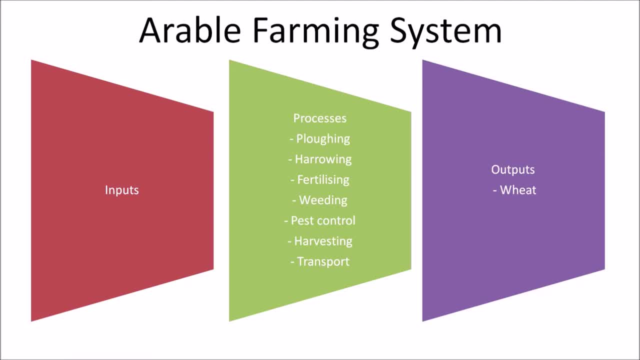 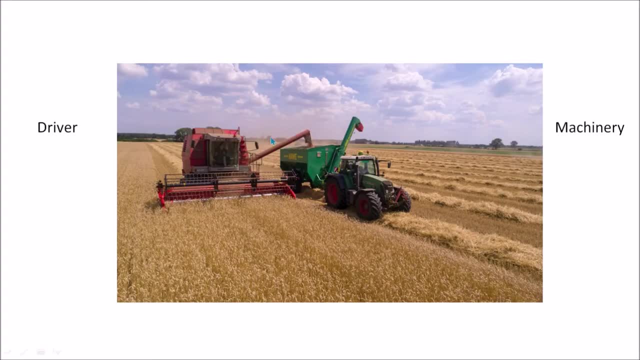 just getting the grains- like getting the wheat out to the people who are going to buy it, So down to the market- you're going to need some inputs. So, even if we just look at the harvest- harvesting with the combine harvester- you're going to need a trained driver who knows how to use these. 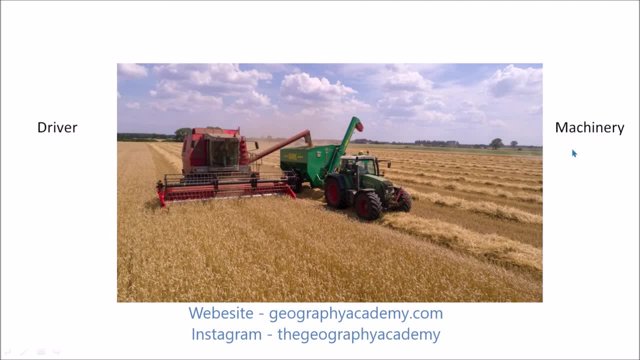 different types of machines and you're going to need to either buy the machinery or possibly rent it. So those are two inputs that are needed there, and you know quite high cost. So instead of having, say, manual labor, which could be cheaper, you have a trained driver. The farmer, obviously, then, is going. 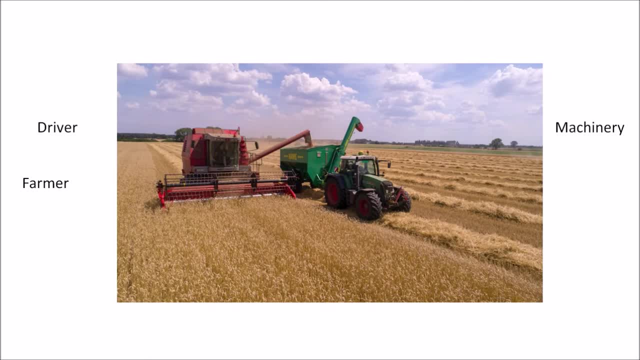 to be an input into this. Now, that can be in terms of someone who grew up there. you could have talked about someone going away and getting a third level education in agriculture, who's then a professional in their field to go out into a farm. But either way, those people are trained. 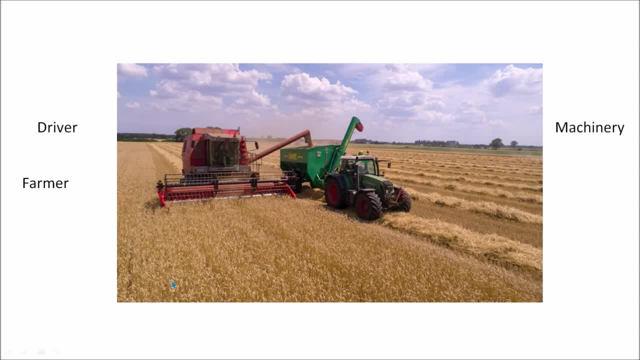 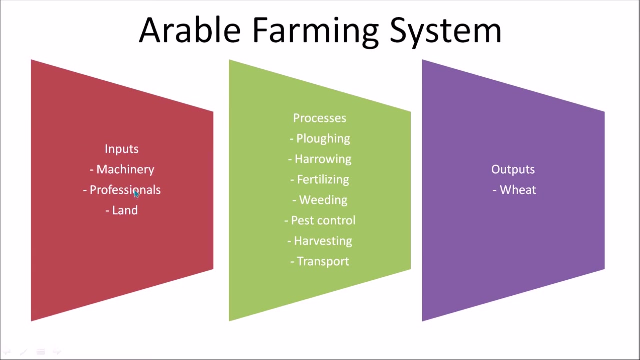 and, yeah, they'll have to be paid accordingly. Then, of course, land- extremely important, So land is needed. so what we're able to take from the land is really what farming is. So, yeah, you need to either buy the land or rent the land, and those would just be a couple of examples of 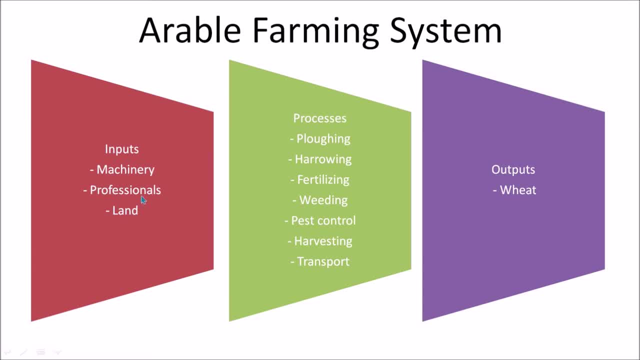 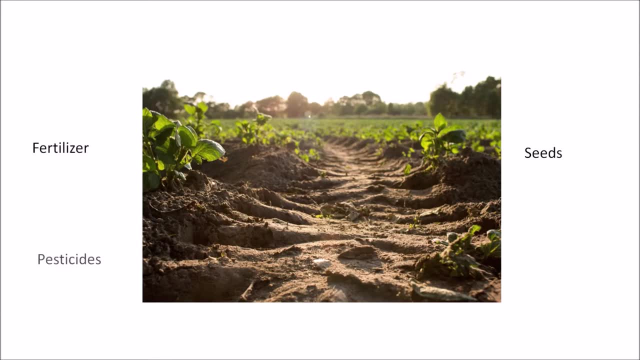 you know what we're able to do- Real essential inputs. So the other things we need, obviously the seeds. We could need fertilizer, We might need pesticides. So pesticides are trying to get rid of anything that we don't want there in terms of like weeds or maybe insects that come along and will actually 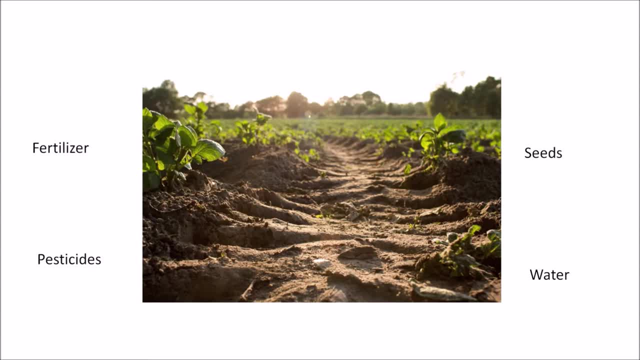 eat our crop. Now you might think, okay, well, if we're in the right climate zone, maybe that's not a huge input, So it rains naturally. So in a lot of countries, yeah, they're going to need to get rid of anything that we don't want there in terms of like weeds or 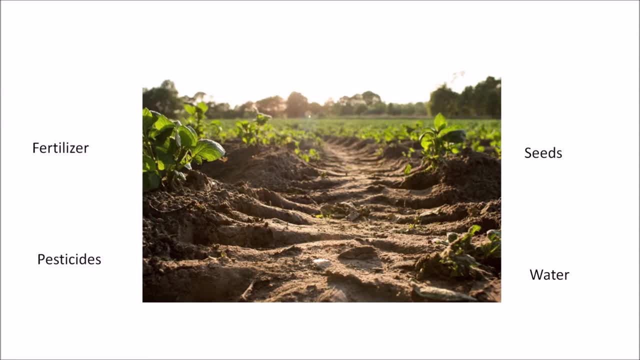 that gets adequate amount of rainfall, This isn't a major issue. However, there's lots of reasons why we might need special irrigation schemes in order to pump the water into the correct area and to utilize the water really, really efficiently. All these things need to be organized beforehand in. 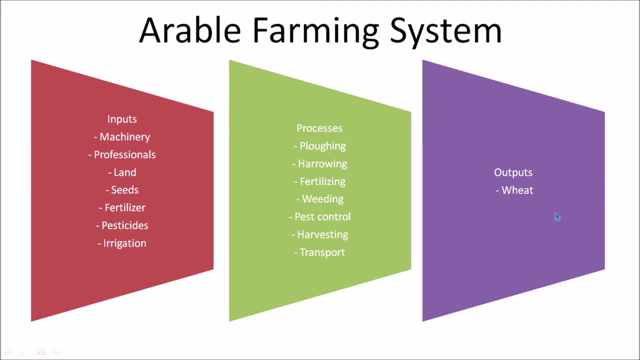 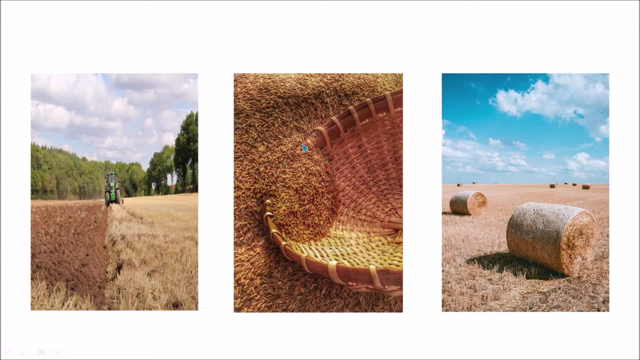 order to actually complete the processes, in order for us to get the outputs. There's lots of different things that we could get from, say, the wheat. We can get the grains. We can also reuse the stalks that are left over. We can get the grains that are left over. We can get the grains that are left over. 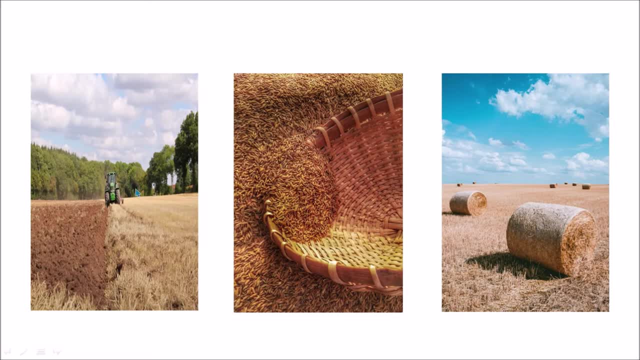 Put them back into the ground to help keep the soil fertile, adding those nutrients and those essential elements back into the soil. We can then take up the stalks, the wheat stalks, and we can use them then later as like feed for cattle, maybe through the winter, when maybe they can't graze. 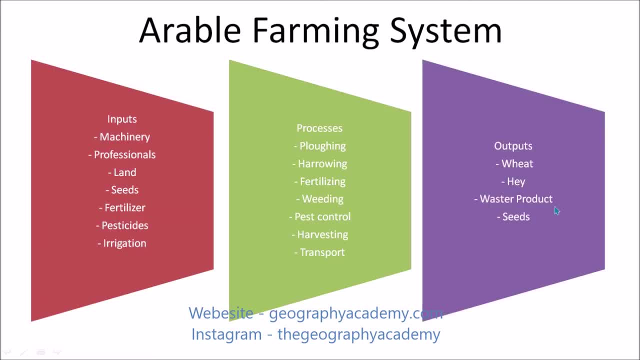 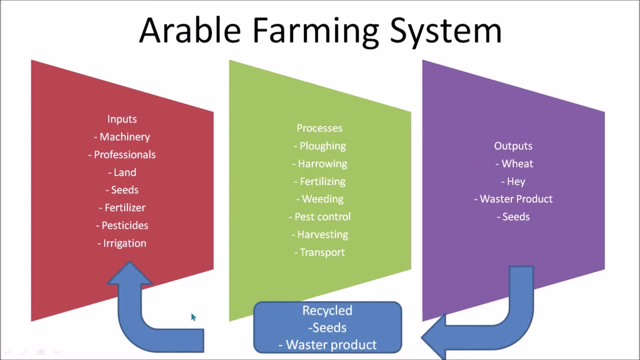 the hay, the waste product and the seeds, So we can use the seeds again in this particular farm Waste product, which is a waste product. Anything that's left over is then going to go back into the system and then possibly the hay, for instance, could be then sent off to a farm that has animals. 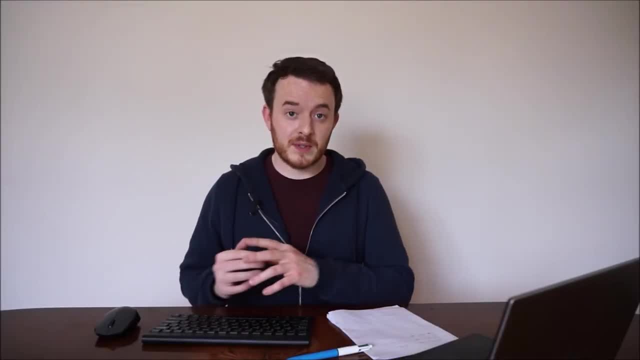 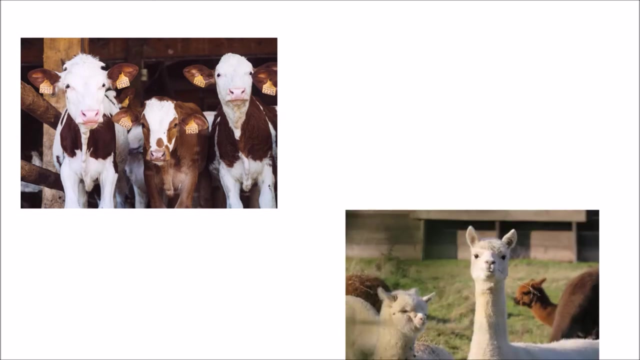 that could use that for feed. So on the other side we have pastoral farming. So in this farming system we see livestock being grown and being cared for in order to produce either and meat or byproducts of that. This will include cattle, cows, maybe llamas, alpacas and sheep. 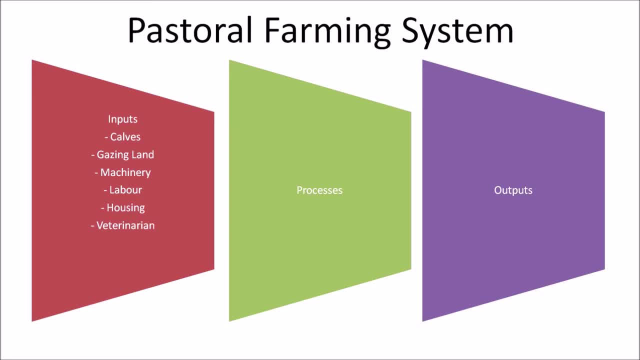 for example, The pastoral system then will be slightly different to the arable farming system. So the inputs, as you can see, we need things like calves, so young animals, We need grazing land, so beforehand you know we need land in order to sow seeds. We'll still need machinery, maybe not on. 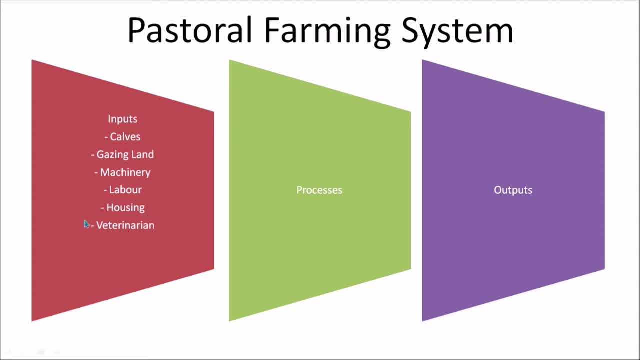 scale. We'll need labor and professionals such as veterinarians, and we'll also need housing as well. So the processes: What kind of things would we be doing? Well, it kind of depends what we want to get out of it. But if we had, say, like a grazing animal, like a cow, we might need to herd the cow making. 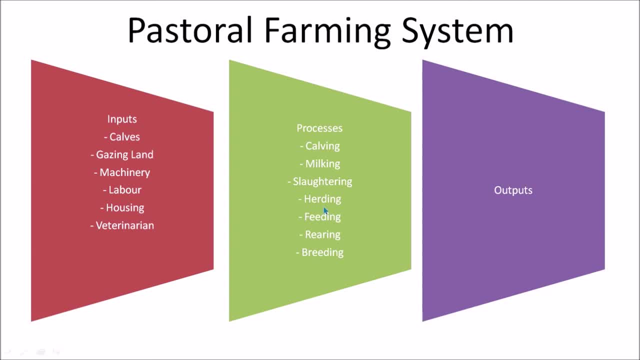 sure that we can bring it from one place to another safely, Make sure that it's fed, that its upbringing is okay and we make sure that it's healthy as it's growing up And then breeding. So making sure there's the next generation of cows to come from that We might use. 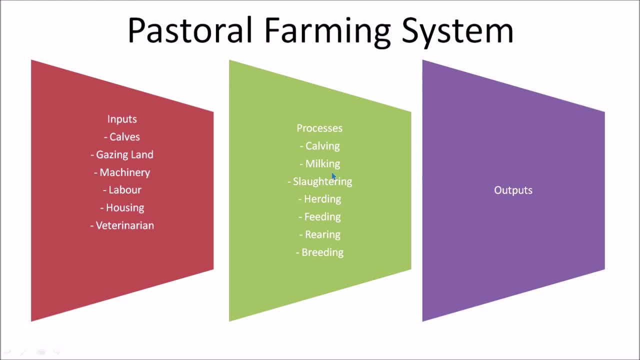 those cows, then, for example, milking, and then we might also slaughter the cows and use them for beef production. So the outputs there could be pretty diverse in terms of, like milk, beef leather. So a lot of animal parts can be used. And then, if you're talking about the recycled system, 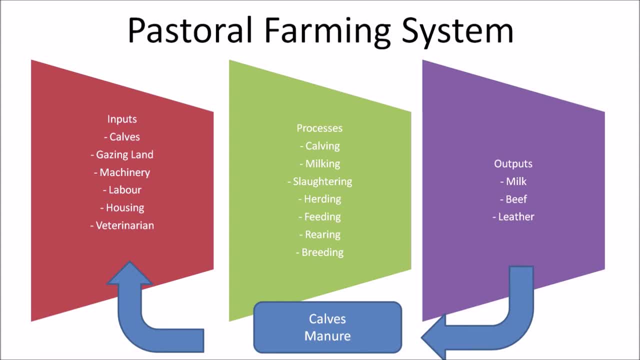 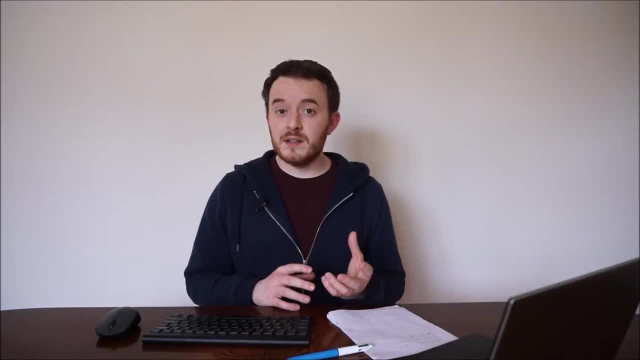 we could say that like the newborn calves, and it could be used, and the manure from the cows could be used to fertilize the soil. like we talked about before, Mixed farming is the combination of both pastoral and arable farming. Now this can be quite beneficial, especially to a farmer who wants to be a little bit more diverse, Perhaps. maybe crops are only able to be harvested in the spring and summer, leaving more money to be made during the autumn, winter, possibly with livestock. Also, you can diversify the type of product you can create, So you could have a dairy. 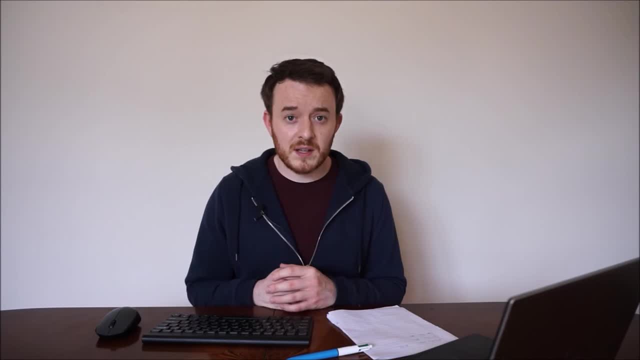 and wheat at the same time. That way, then, you have two sources of income, and if one fails, the other might be able to keep it afloat. The other benefits of having a mixed farm is that, of course, you can use some of the recycled products for other uses, So having a waste material that could be used as 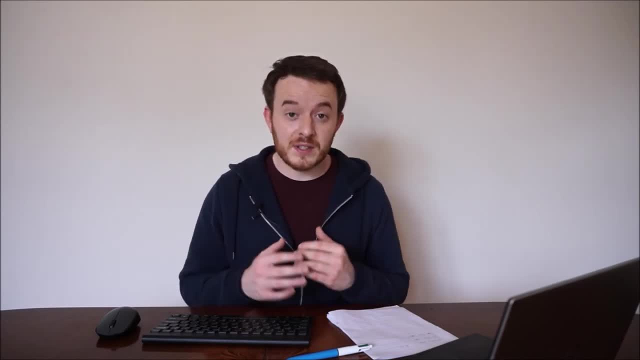 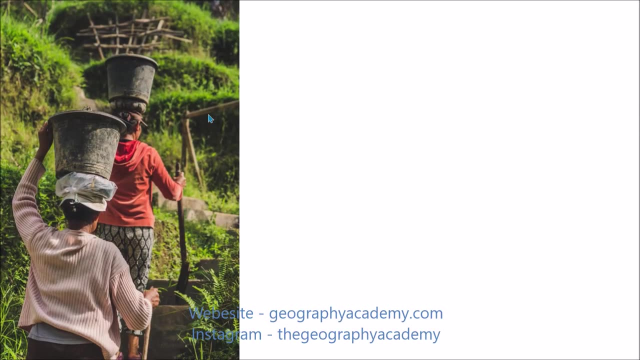 food for the animals during the winter is highly productive, meaning that there's less waste on the farm and that you can get the most out of your own product. Persistence farming is farming to meet the needs of you and your family. So if you're a farmer and you want to make sure that you're 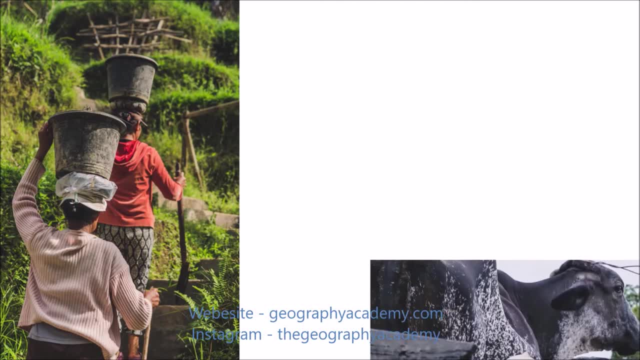 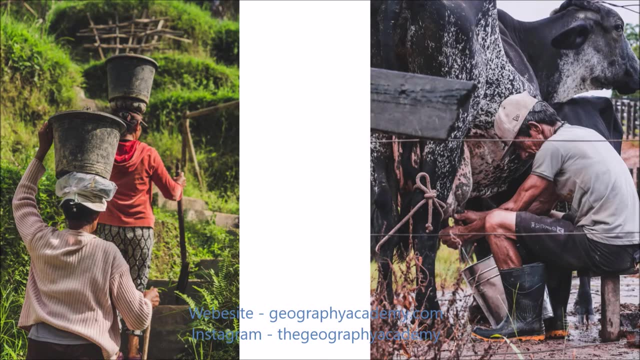 getting the most out of your family. So oftentimes we can see this as being quite small scale, possibly within the family. The technology may be quite low and quite basic. We'll see maybe a low input of capital and then we might have like less in terms of the input in like plants and animals. 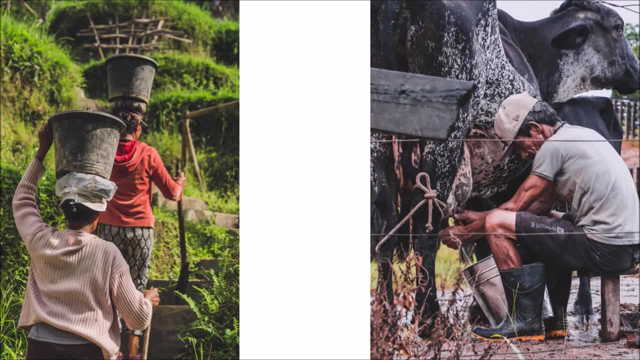 So oftentimes, whatever's produced in a subsistence farm is usually actually consumed by the family unit, or possibly the family unit itself. So if you're a farmer and you want to make sure that you're getting the most out of your farm, then this may be an option And, lastly, there's a small amount set. 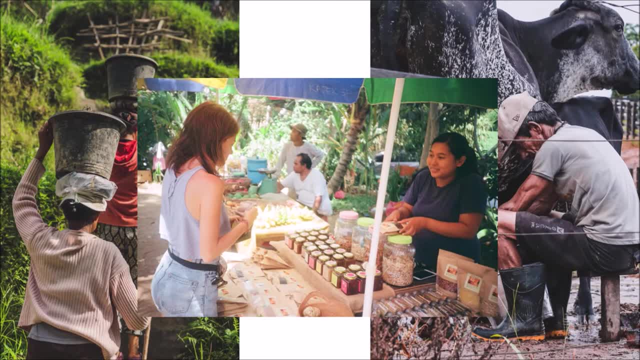 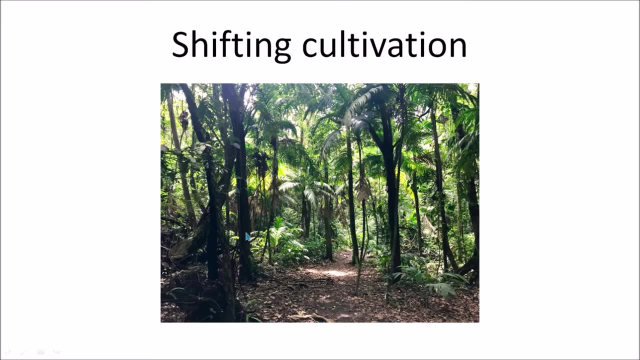 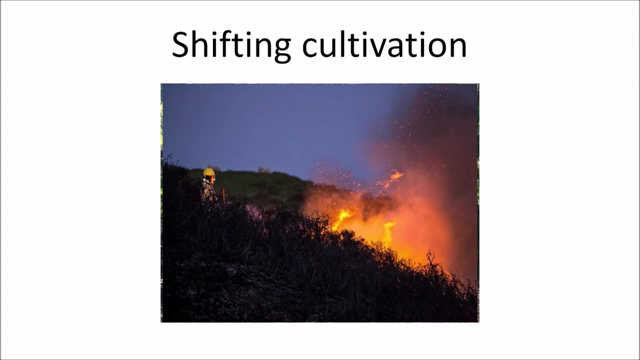 off for profit, just to make sure that you can have money to maybe diversify your diet. So this could be done in a small scale as well, maybe like local farms and local grown products. Shifting cultivation is an example of this, where an area of forest may be stripped down, cut down and then burnt. 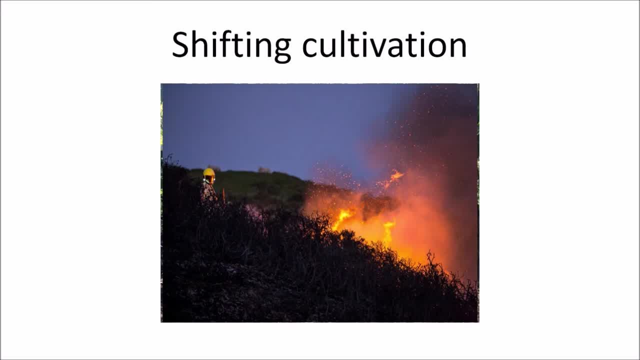 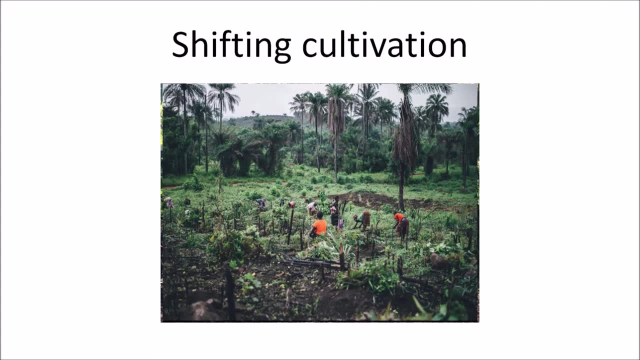 And this would be a slash and burn technique. So the burning then allows for all the good nutrients to be added to the soil and to make the soil quite fresh. So this is something that we're looking to. fertile for a short period, This area is then planted and farmed, so it might be turned into. 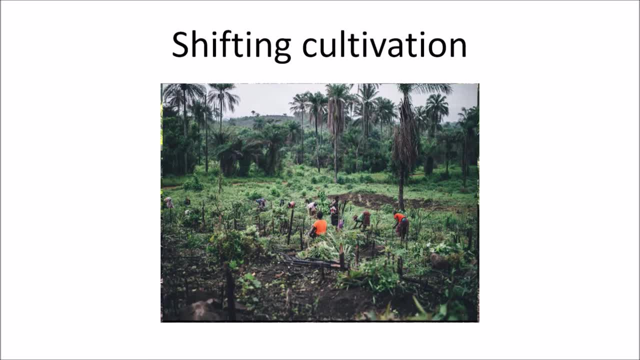 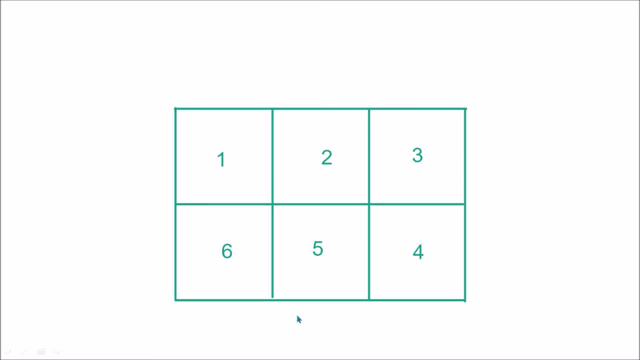 like here, an arable farm, but you may also have like animals grazing in the area too, and then you can also forage in the local area. So this would be an example of shifting cultivation. Now the idea of shifting or moving is that they would start off and maybe plot one here. 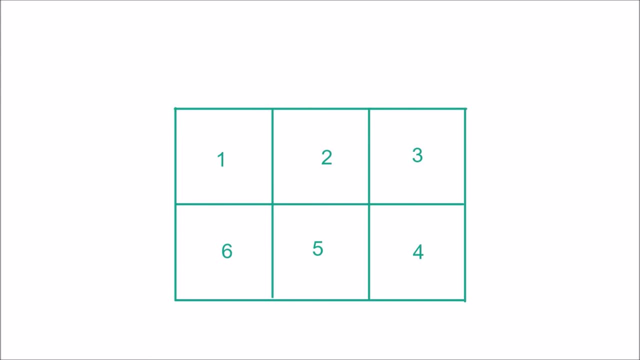 they would cut down all the trees and the plants here and then they would burn them, grow the plants or the crops and then after a couple of years the actual like nutritious value and the fertility of the soil, I should say, is going to be gone. so they need to move on, So they 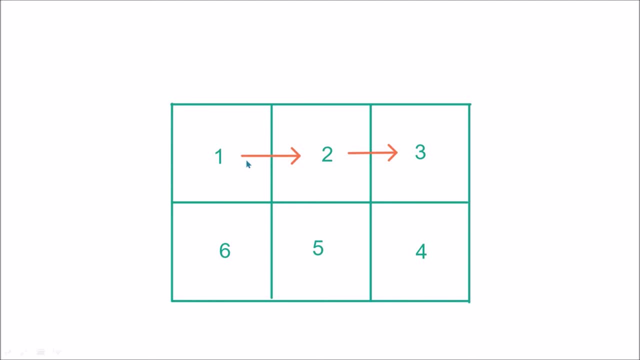 go and cut down the next area and continue on in that fashion. Now, while they're going around to the second part, the first area, the first plot of land gets a chance then to recover. so after about 10 years they've then moved between plot one and plot two, and they can go on to plot number three. 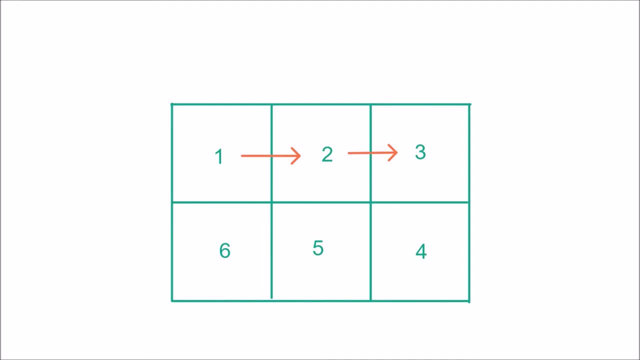 And in this area then it continues. so number one has now had 10 years to say, recover. if it was a five-year period on each one and by the time they're finished on three, it's had 15 years to recover, allowing a lot of the, the forest to grow back, but not fully mature, But after maybe 25 years 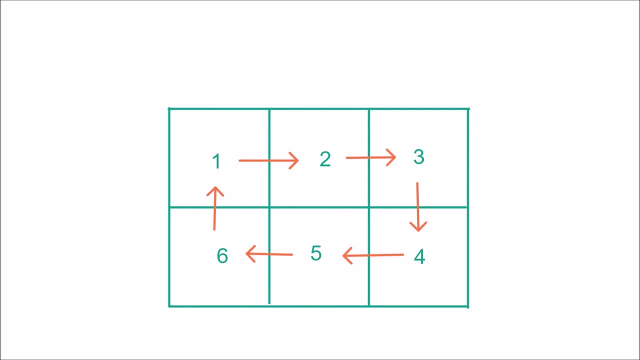 or 30 years. then it has a chance to go through that process again. So that would be shifting cultivation, which is fine. in areas that might have small populations broken into different communities, They can use the land and make sure that it has a chance to regrow. Now this is becoming less and 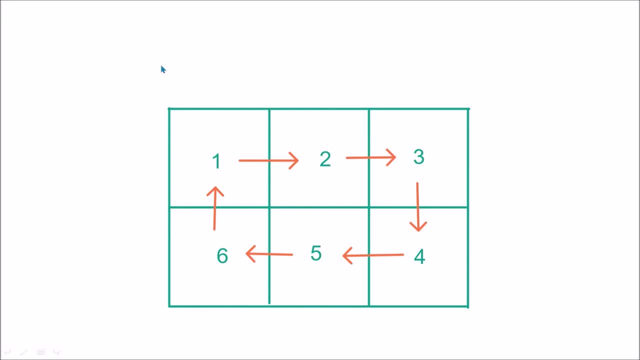 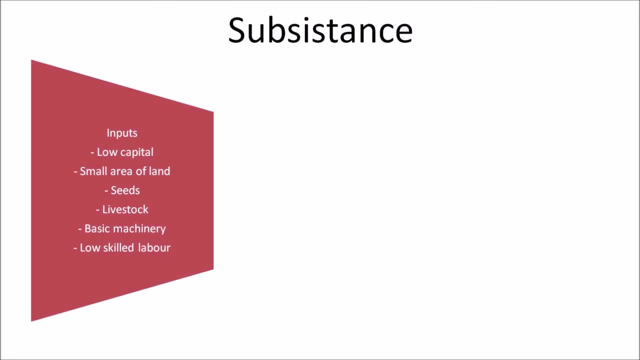 less frequent. We do see it in areas that have quite a tropical climate and dense areas of forests like such as tropical rainforest. So in subsistence farming our inputs could look like this: We would have low capital, small area of land. We'd have to have seeds and livestock. 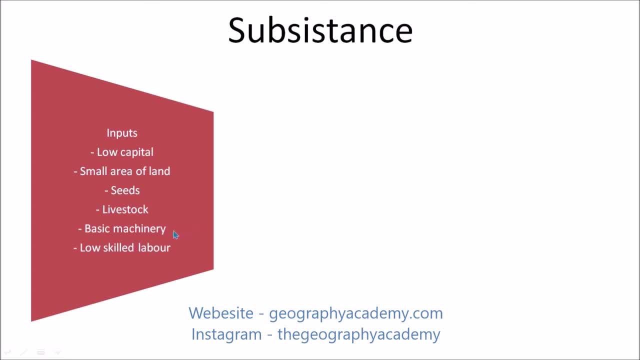 anyways, but maybe on a smaller scale. They would have like basic machinery so you might have. for instance, it's common to see like a plow with something like a water buffalo, where the buffalo is dragging the plow and the person standing behind it Meaning that it's low. 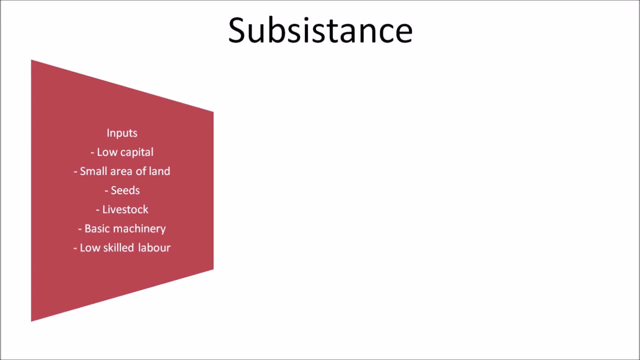 cost to actually buy a simple plow like that, but also it doesn't take great knowledge or understanding to repair it. So low skilled labor oftentimes- or at least it's passed down with generation- There's nothing got to do with. maybe huge machinery that might require, like an. 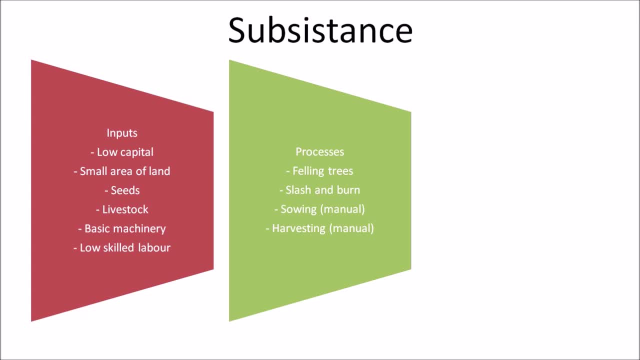 engineer Processes, then they have to cut down the trees or the felling the trees and the slash and burn process. then sowing and harvesting can often be manual, and also, you know, the other things that we talked about, like rearing chickens, for example. Outputs of that may be a kind of diverse range. 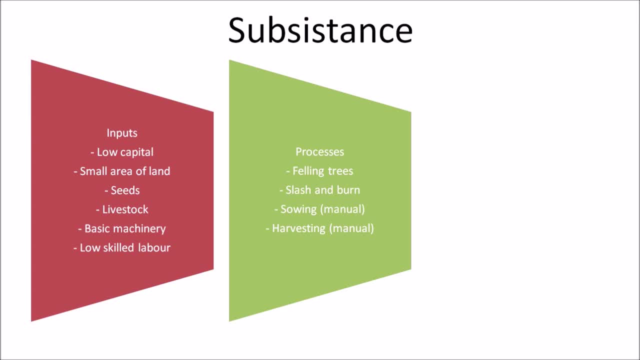 of meat, vegetables, fruits and grains and you know that would cause the family unit to be able to have like food throughout the different seasons. They may sell off some for a little bit of money and they may use the seeds from the plants then on young animals to try and rear, maybe to sell on. 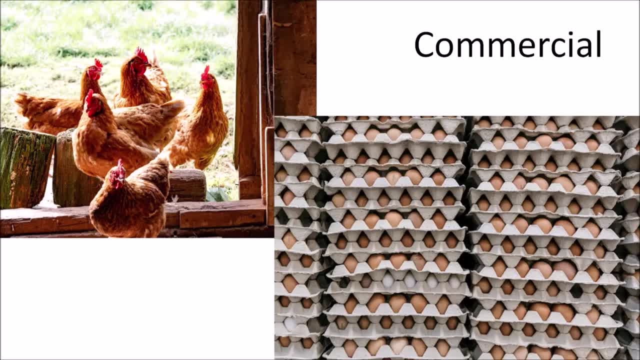 or maybe to put back in and recycle into the system Commercial farming. you want to be making profit and that's what you're going to live off, not really what you produce. So on that you could create like a monoculture, like, say, rearing chickens for the production of eggs on a mass scale, to try. 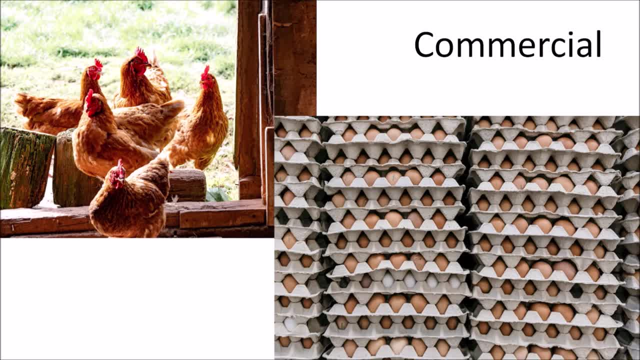 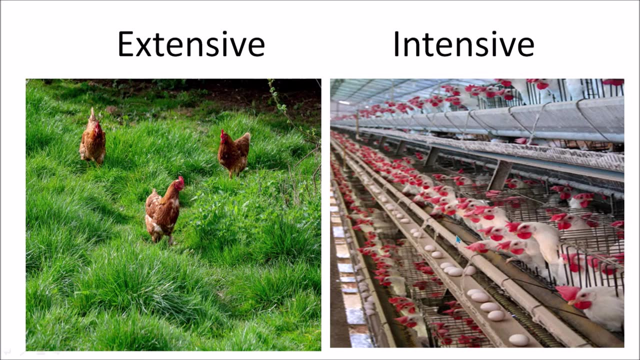 and produce profit, Then if the farmer is, you know, quite a small scale farmer, they can use that profit to support their family, So that's a good thing. They can then use it to maybe build a business and develop from there. So with any farming you would find that they can fall under the categories of intensive or extensive. So if it's intensive, it means we're making the most out of the space, So this might require higher amount of capital. Now, using the chickens again as examples, we can see here there's not much space for these chickens and they're in tiered rows, meaning that they're out of space. So that's a good thing. 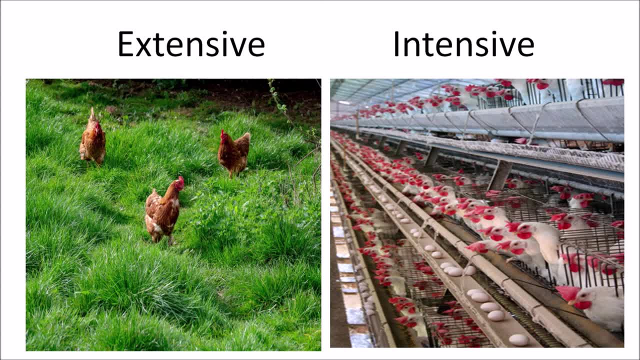 They're not confined within that region, but the area of land is used to the maximum capacity. So these chickens will actually stay in this area. You can see they feed here. The eggs are brought down through there and they're kept in this captivity. So for this one here it's a very intensive process, with high profitability then and maximizing the use of the land, Whereas the chickens over here on the left have some land to roam around in and they'll lay eggs then. 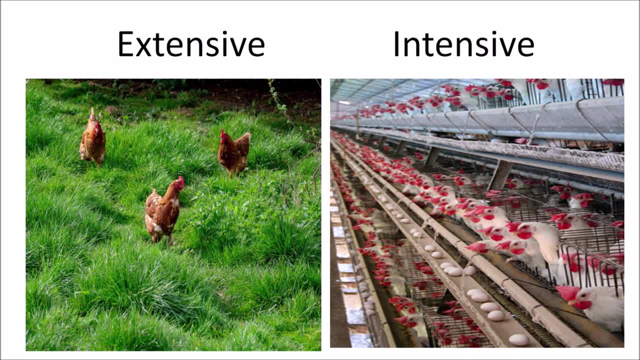 In a particular area. Yeah, so this will be more extensive in the fact that it's a huge area of land and not many chickens. Now. the same can be said for any type of crop. How do we use the land, And we'll go into that in a bit more detail in the next video, And as well with like rearing cattle and what are good practices and sustainable practices. But as long as you have a fair idea of the difference between intensive and extensive subsistence and commercial farming, you should be good for this. 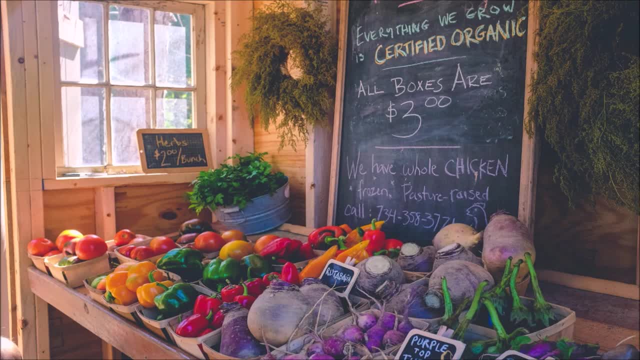 So let's take a look at this video: Three, Two, One And go. So to introduce the idea. we always see these labels in shops: organic, inorganic, Okay, start again. Three, Two, One, Go. So we often see this now coming up. so things here: Everything we grow is certified organic. 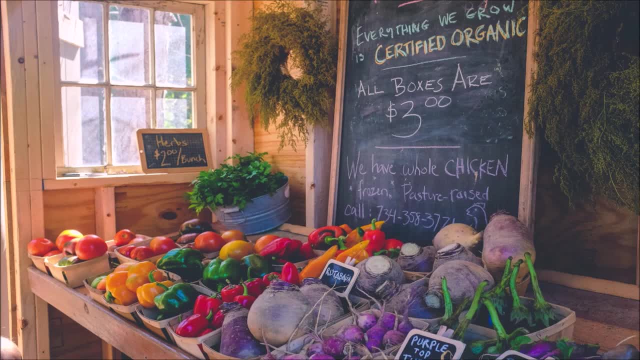 So what does it mean to be organic? Well, the idea of an organic farm is that you're not using manufactured or like chemically produced products to help grow your crops or to help rear your animals. It's a natural environment. So an example we used earlier was how to look after the soil. 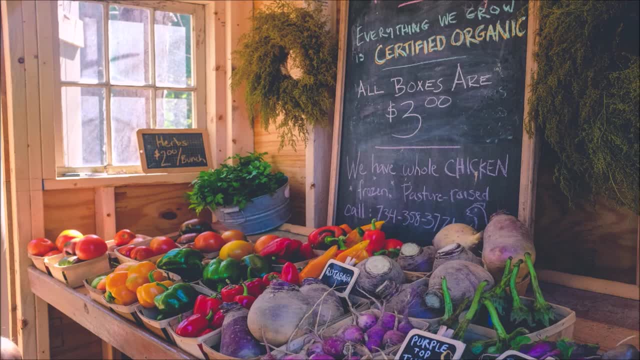 You could, for instance, use manure as like a natural fertilizer, or you could buy bags of chemically produced fertilizer. The chemically produced fertilizer is then going to Create So the chemical fertilizer are then going to aim for the specific needs of the plant. 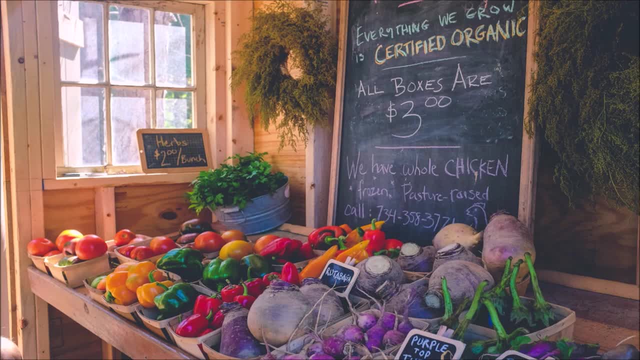 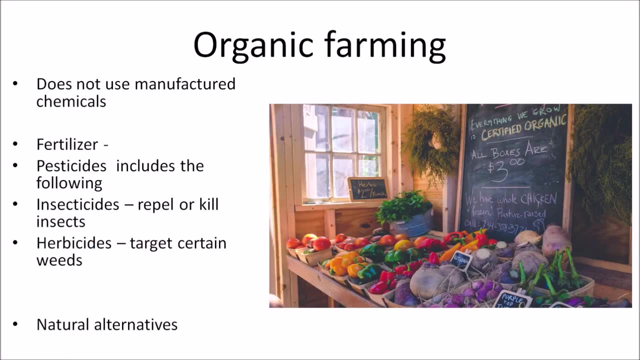 And this is going to help the yield of the field increase, So we're going to get more out of that. So yeah, apart from not using the chemicals- certain ones they're going to stay away from, So like insecticides to repel or kill insects, or herbicides- 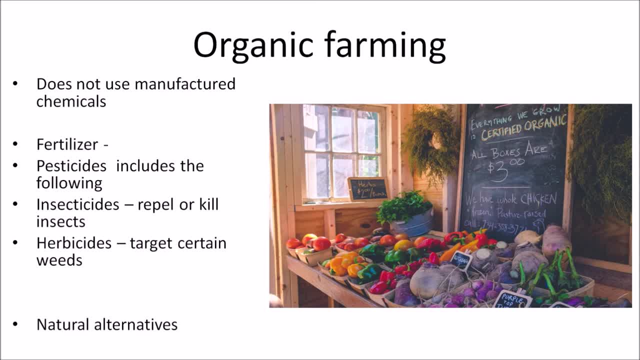 These kind of like target the weeds that we were talking about earlier, So we could find natural alternatives. For example, with the insecticides We could find natural predators For the insects that could be eating the crops And by that way we like create a natural ecosystem and create a balance within that area. 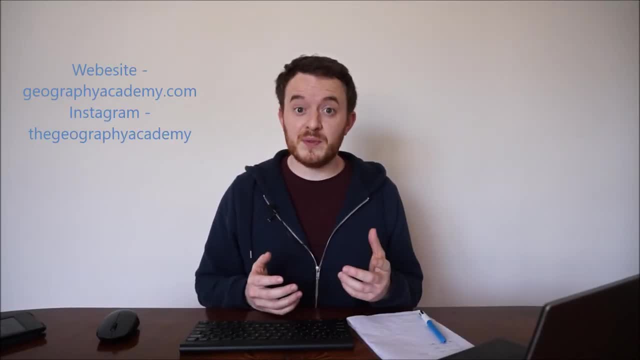 Okay, so that's the end of the video. Thanks for watching. I really hope that was helpful. If you want the notes from that, you can come over to thegeographyacademycom. Link is below. Also, if you want some help answering exam paper questions and with the exam paper skills, 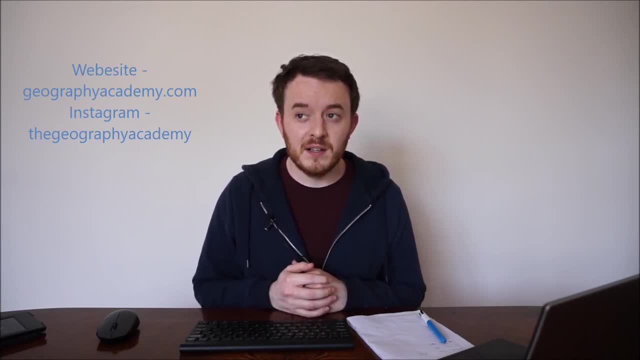 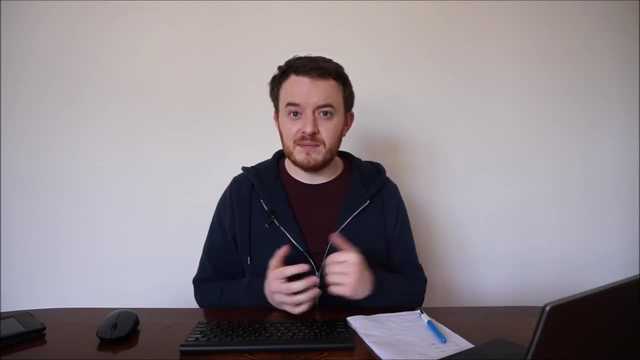 Go over to Instagram And we'll be setting up some updates there Once we get some followers on that. So hope to see you soon. And yeah, like subscribe and all that sort of stuff. Thanks.